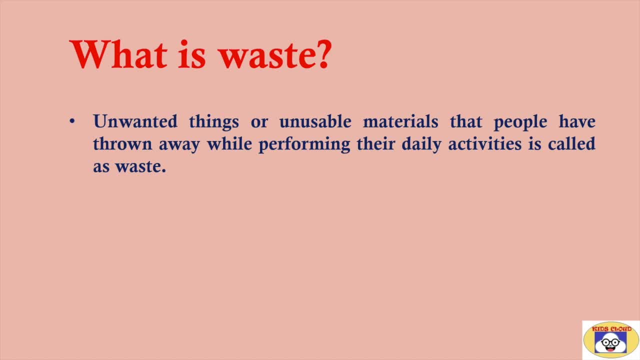 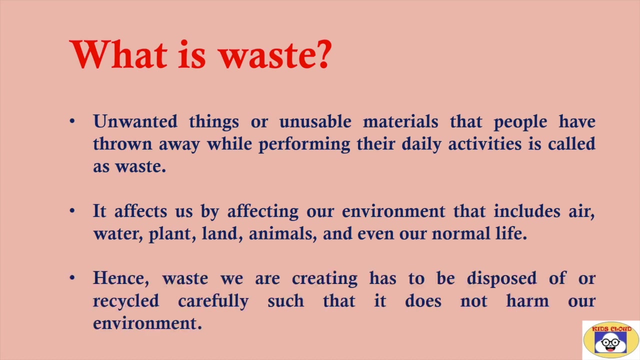 that people have thrown away while performing their daily activities is called as waste. It affects us by affecting our environment. that includes air, water, plant land, animals and even our normal life. Hence, waste we are creating has to be disposed of or recycled carefully. 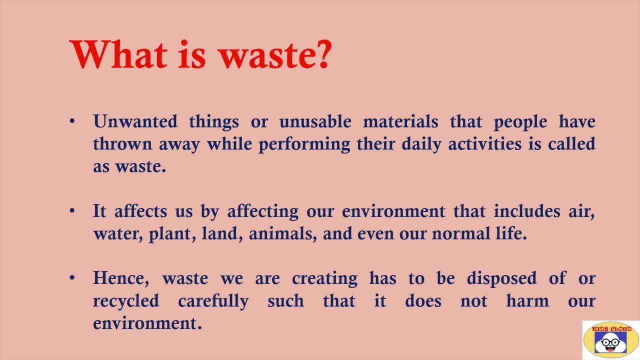 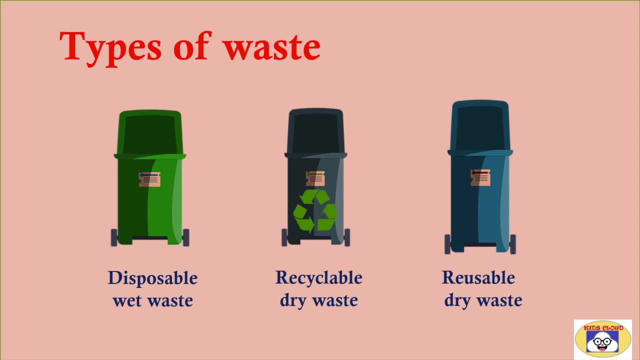 such that it does not harm our environment. For simplicity, we can differentiate the waste generated at home into three different types: Disposable weight waste, recycled waste, recyclable dry waste and re-usable dry waste. Now, what is this disposable weight waste? 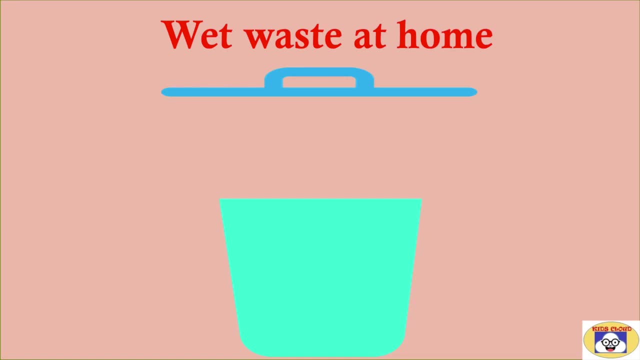 We can enlist some of the things that are generated at home and we can consider them as weight waste. Weight wastes mainly include fruit peels, vegetables, spoiled food, cooked food, uncooked food and flour waste. This is biodegradable waste and we have to dispose of it properly. 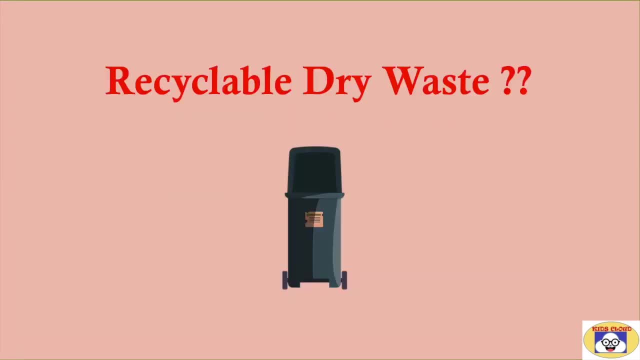 Now, which is the dry waste that is generated at home. This mainly include wooden waste, newspapers, magazines, packet wrappers, packaging, waste paper, packaging bottles, paper and paper bags and other items that are made with recycled waste. This is mostly used in various jobs, which may include Paris. 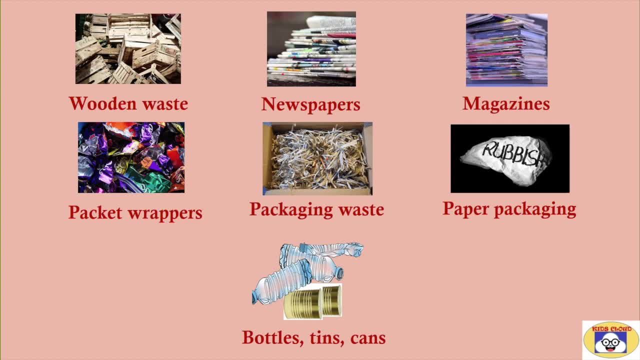 This is commonly used in the process of recycling waste and packaging waste. This is mostly used in organic waste, as well as in wetter waste and other waste: bottles, tins, cans, etc. This type of waste need to be recycled properly. 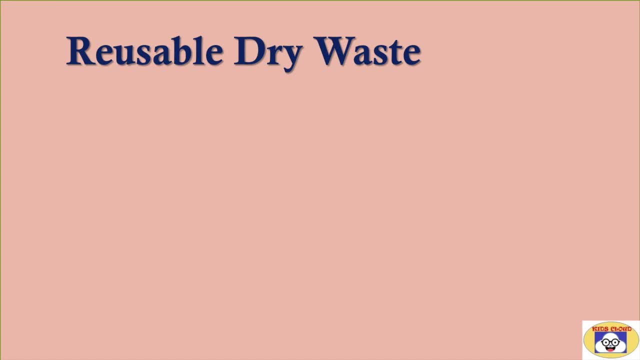 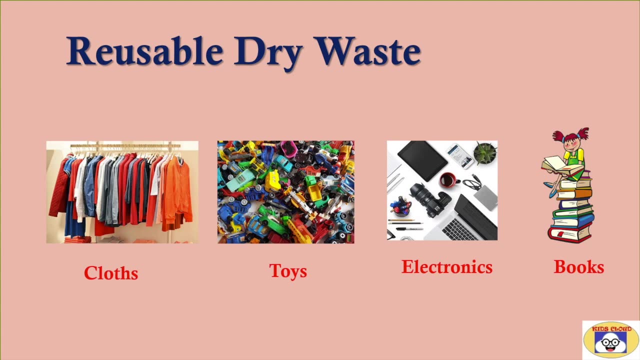 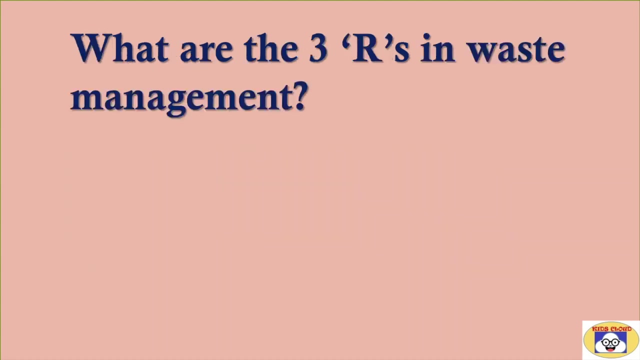 Third type is reusable dry waste. We can reuse certain things, which include clothes, toys, electronics, books, etc. The waste generated at home can be minimized by following three R's. These are reduce, reuse and recycle. Reduce means refuse to buy items that you don't need. 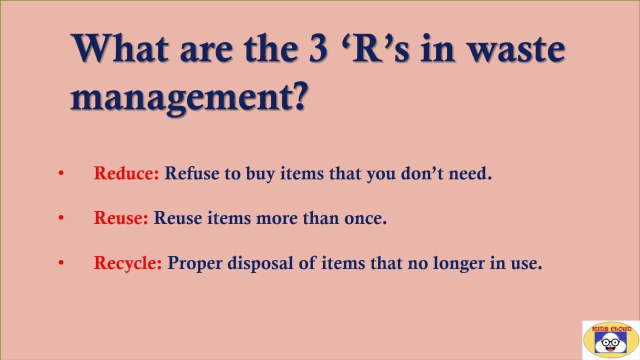 Reuse means reuse items more than once instead of throwing them, And recycle means proper disposal of items that no longer in use.